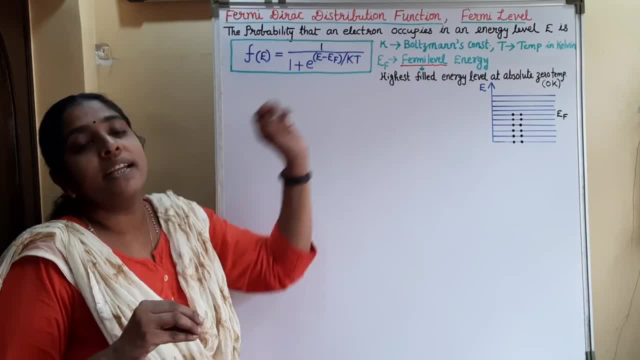 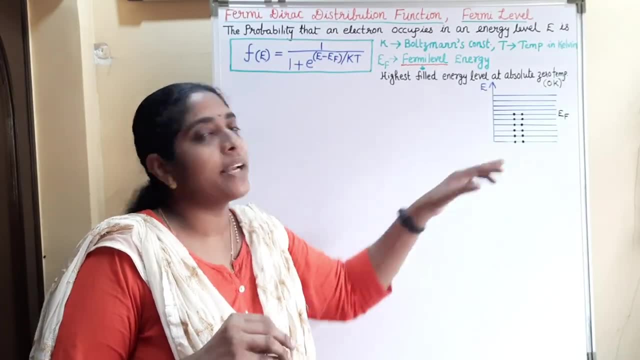 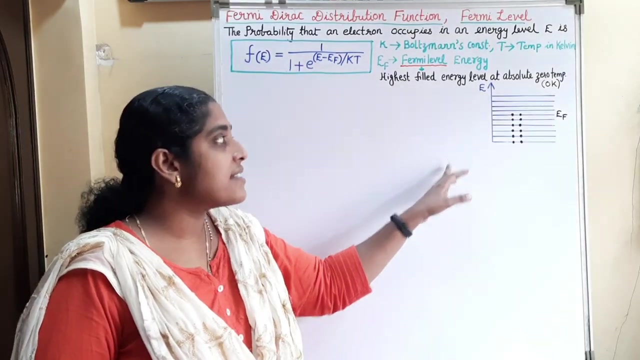 K is the Boltzmann constant, T is the temperature in absolute scale, that is in Kelvin. So here the lower energy levels are filled in this diagram. That means the probability of occupancy of electron in these energy levels are 100 percentage, Whereas the upper energy levels 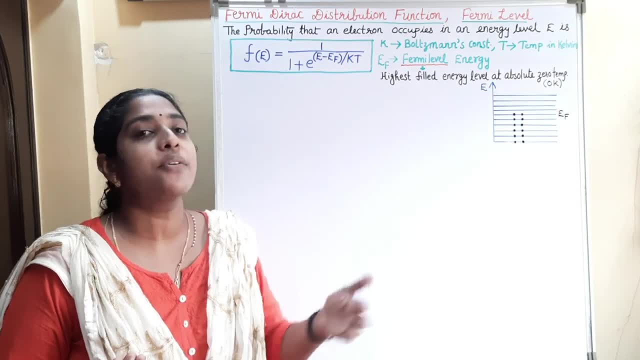 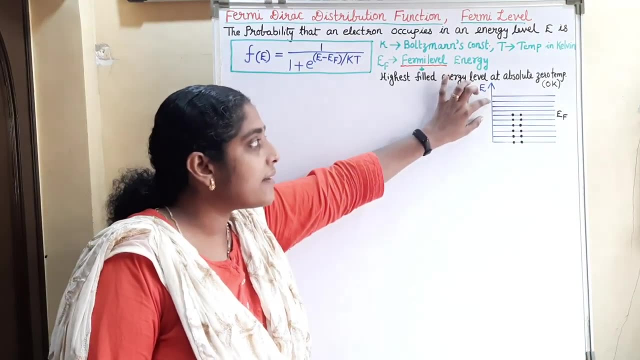 are empty. That means the probability of occupancy of electron in the upper energy level is 0 percentage. So Fermi Dirac distribution function will be 0 for the upper levels and 1 for the lower levels. Now we can see more about the Fermi energy in the Fermi Dirac distribution. 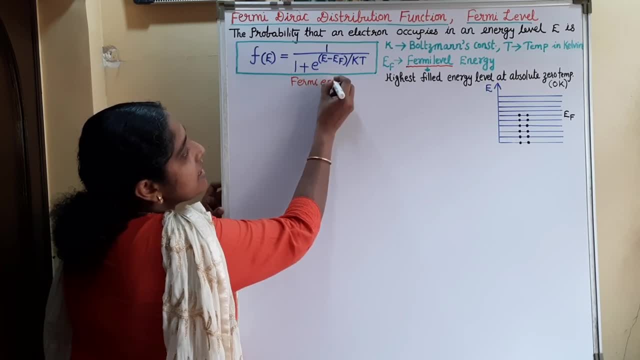 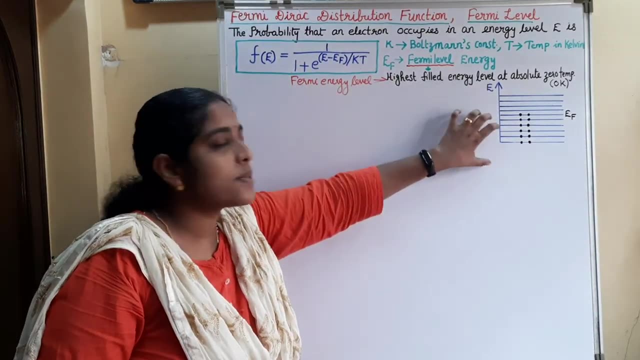 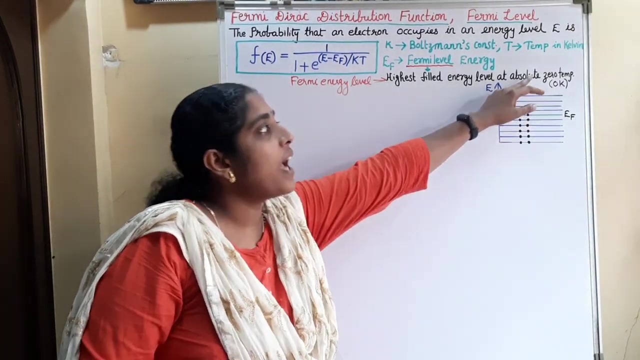 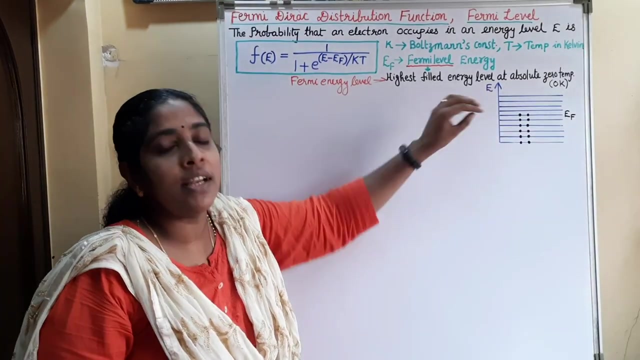 So what is this Fermi energy level? Fermi energy level is a reference energy level that is used to specify other energy levels. It can be defined as the highest filled energy level at absolute zero temperature, That is, at zero Kelvin. At zero Kelvin the uppermost filled energy level is known. 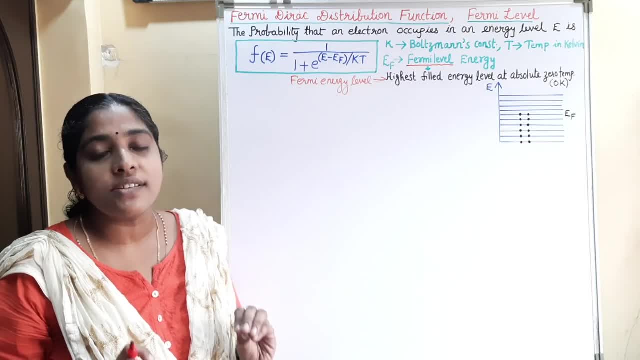 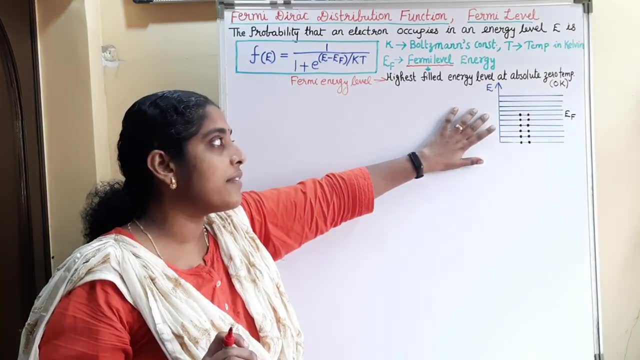 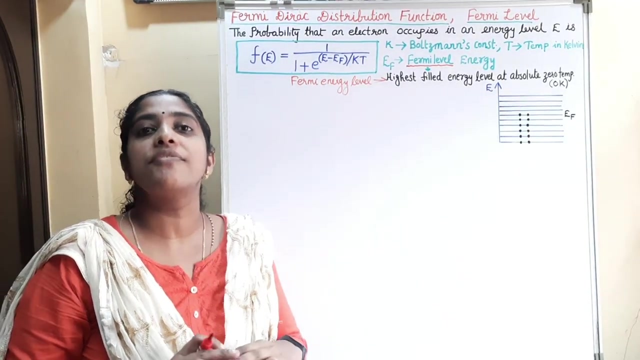 as the Fermi energy level and the maximum energy of the electron is 0. So Fermi Dirac distribution of electron at zero Kelvin. that is the Fermi energy, That is, all energy levels above Fermi level are empty at zero Kelvin and all energy levels below the Fermi level are filled at zero Kelvin. 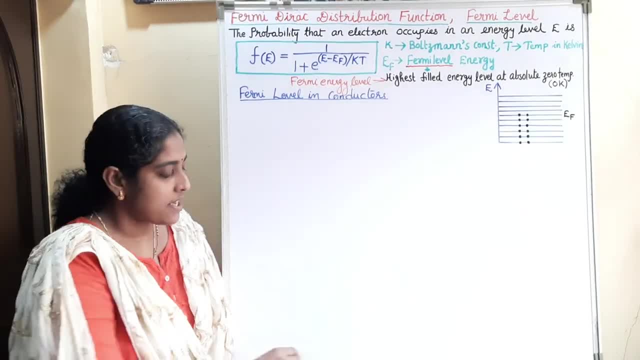 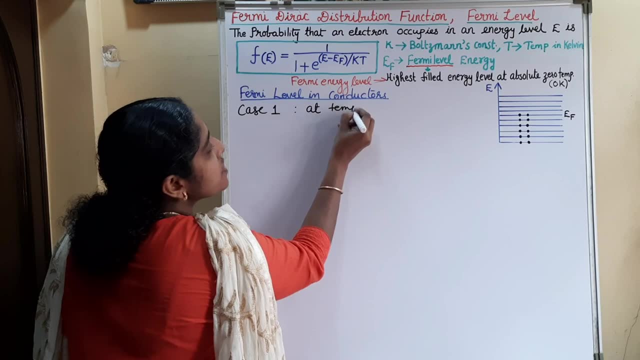 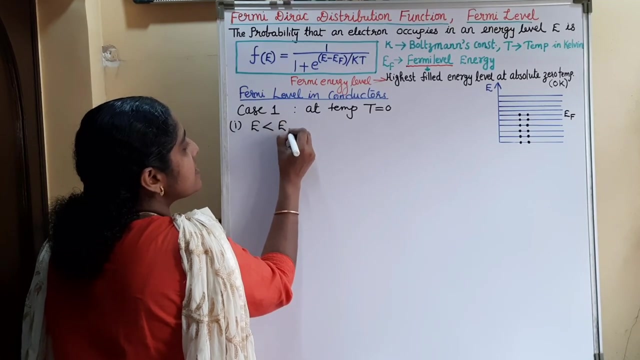 Now we can see the Fermi level in conductors. So first we can take the condition at temperature T is equal to zero. So here the first case is: if E is equal to zero. So here the first case is: if E is less than EF, That is, we are considering the energy levels below the Fermi energy level. So if 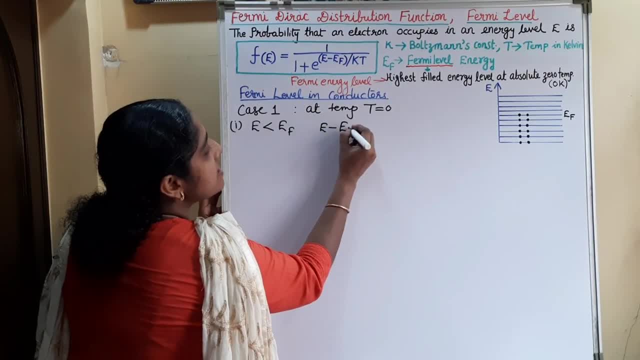 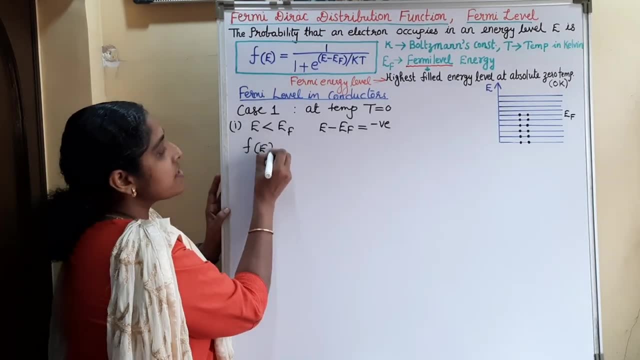 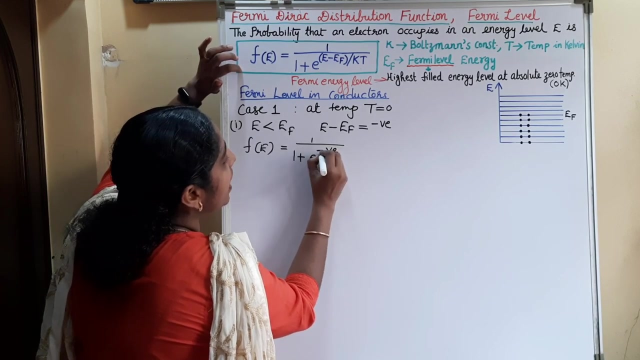 you are considering the energy levels below Fermi level, this E minus EF is equal to negative. So while we are considering the Fermi Dirac distribution function, it is equal to 1 by 1 plus E. raised to negative value. divided by K into K is Boltzmann constant into T, That is T. here we 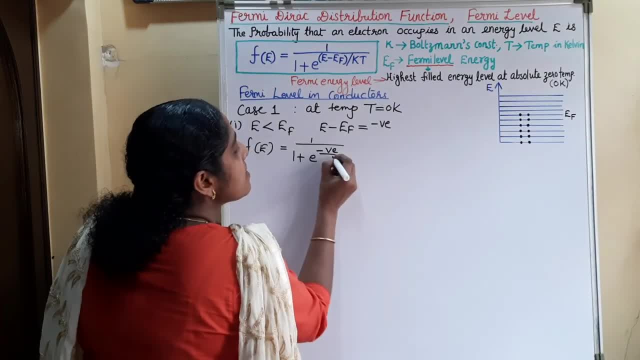 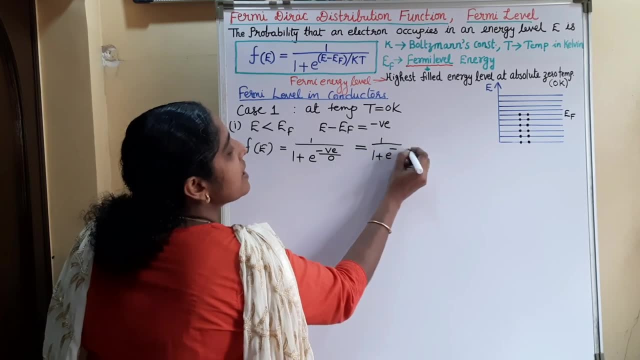 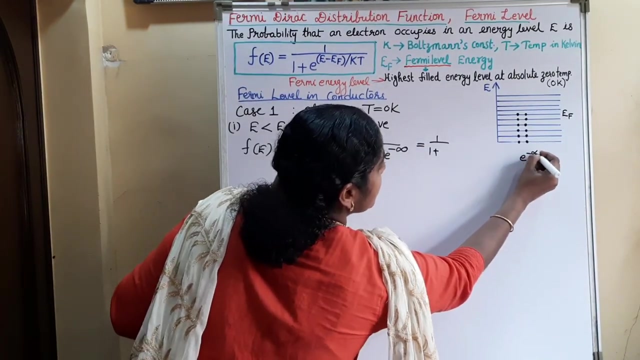 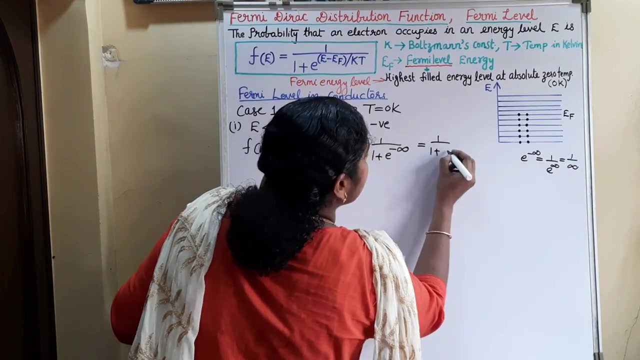 are considering the case of zero Kelvin, So here this becomes zero. So that is 1 by 1 plus E raised to minus. a value divided by zero is infinity. That is 1 by 1 plus what is E raised to minus infinity? That is 1 by E raised to infinity. E raised to infinity is infinity, So 1 by infinity. 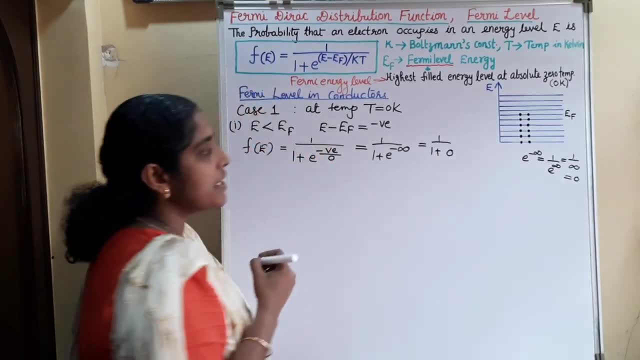 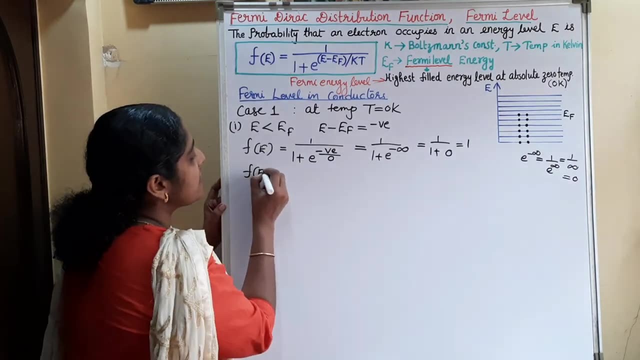 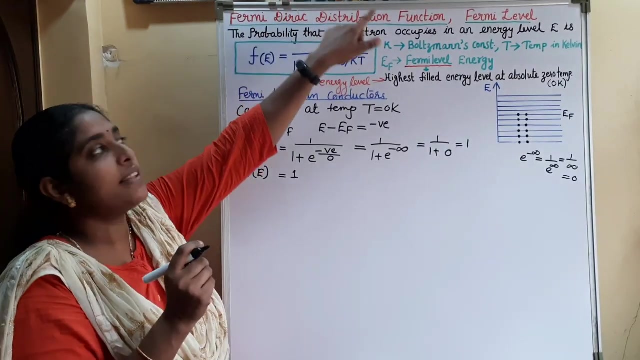 is zero. So E raised to minus infinity is zero. So 1 plus 0 that is equal to 1.. So what is the meaning of Fermi Dirac? distribution is equal to 1, that is, it is corresponding to 100 percentage, So 100 percentage probability that electron can. 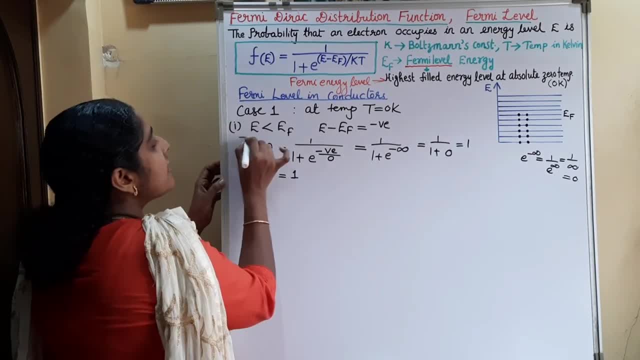 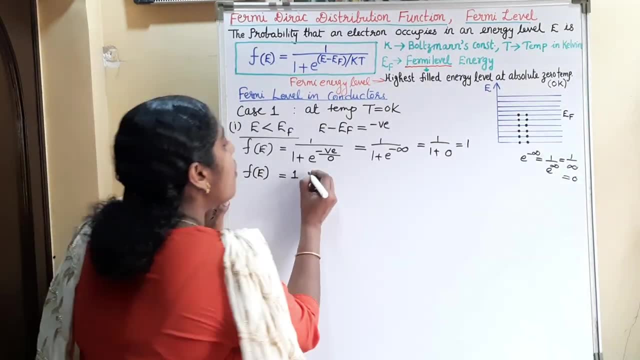 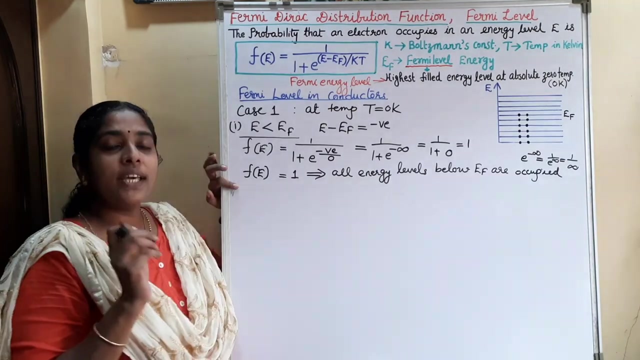 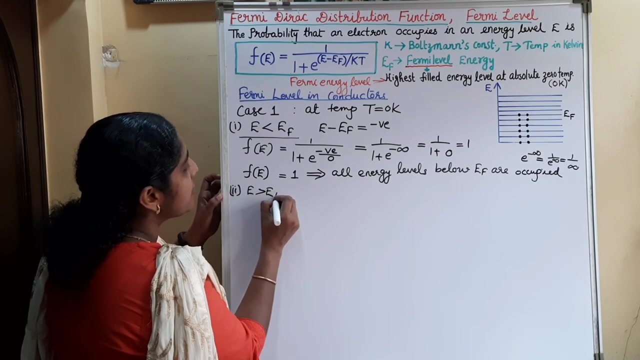 occupy in the energy level if we consider the energy levels below the EF. So here the probability distribution function equal to 1 means all energy levels below EF are completely occupied. Now we can consider the energy levels above EF. that is E greater than EF, So in this case E minus. 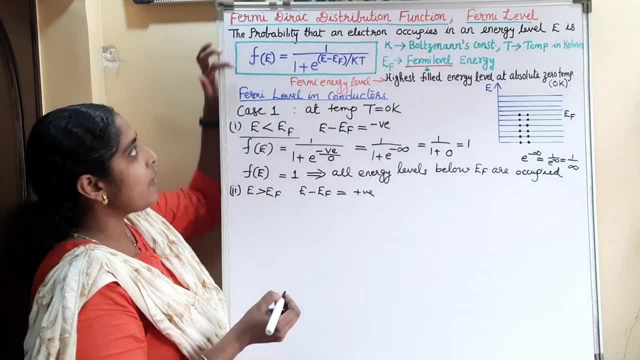 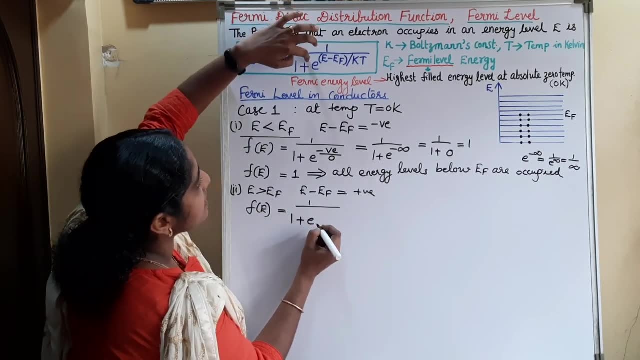 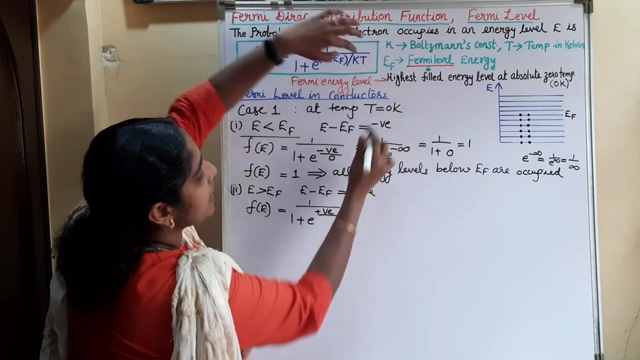 EF is equal to a positive quantity. So what will be our Fermi function? that is equal to 1 by 1 plus E. raise to that is exponential. E minus EF, that is a positive value. divided by Boltzmann constant into T equal to 0 Kelvin, that is 0. 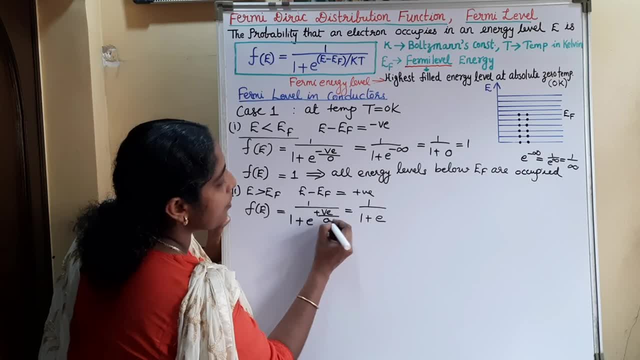 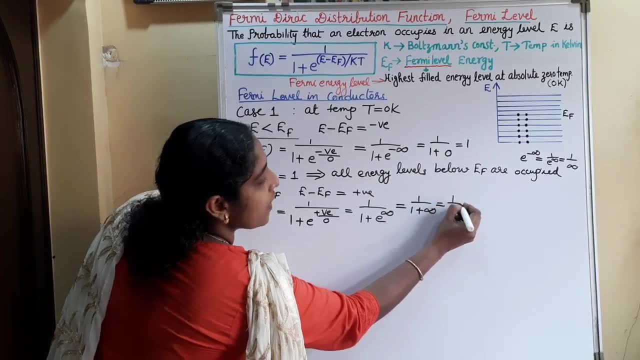 That is 1 by 1 plus E. raise to a positive number by 0. that is plus infinity. So 1 by 1 plus E raise to infinity is infinity. that is 1 by 1 plus infinity is infinity. So 1 by infinity is 0. 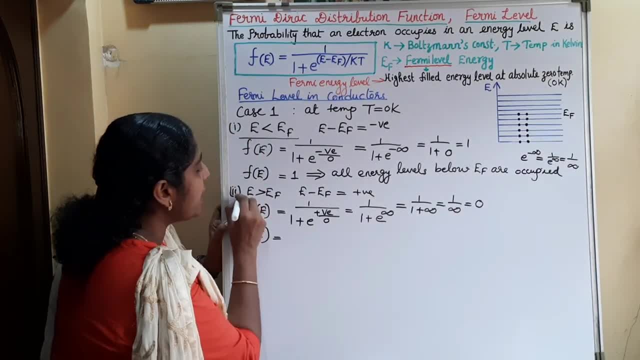 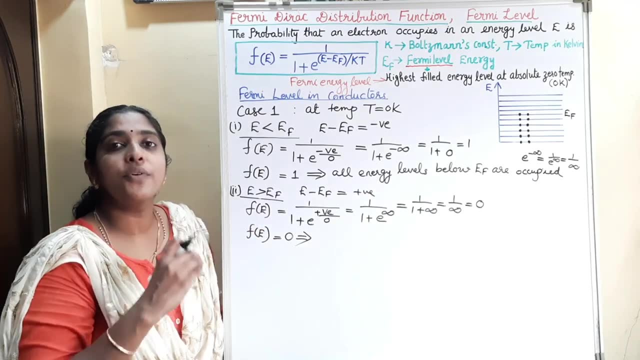 that is Fermi Dirac distribution function for E greater than EF is 0.. F of E is equal to 0 means the probability of occupancy of electron in the energy levels above Fermi level is 0. So this is: the probability of occupancy of electron in the energy levels above Fermi level is 0.. So this is: 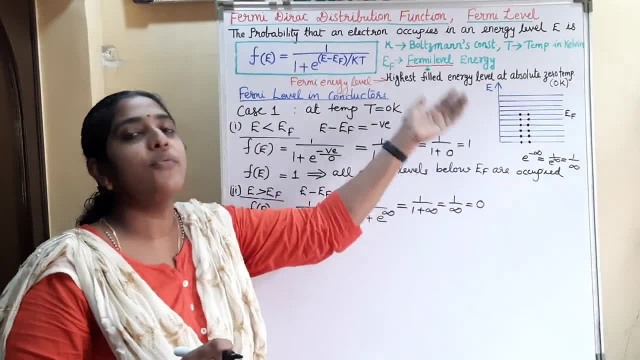 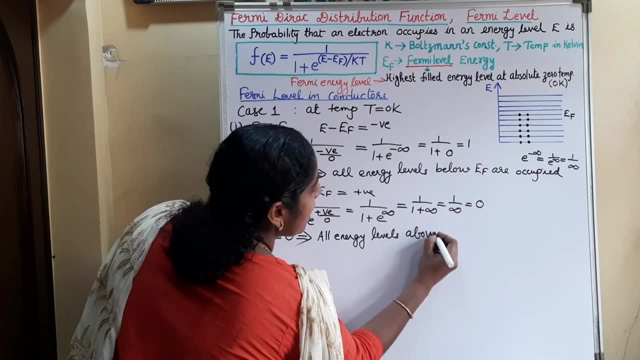 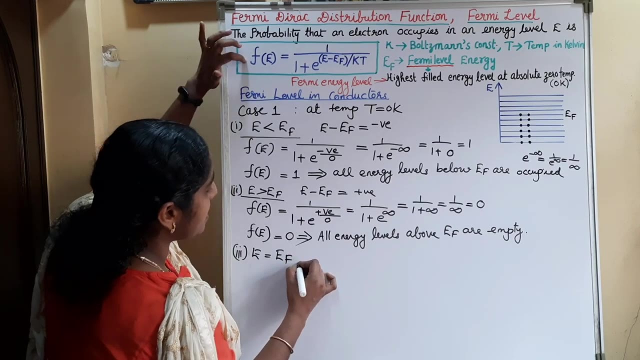 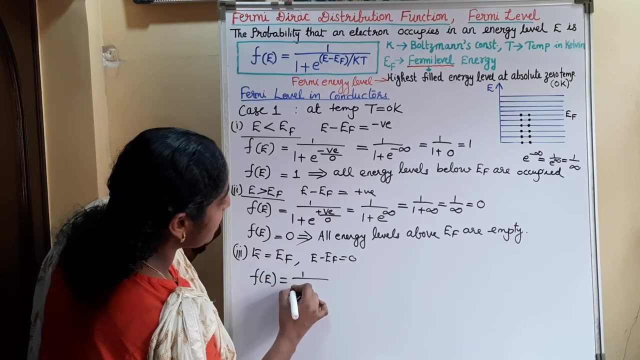 0 percentage. That is, all energy levels above Fermi level are empty. So that is, all energy levels above EF are empty. Now we can consider the last condition. E is equal to EF, So that means E minus EF is equal to 0. So what is F of E? F of E is equal to 1 by 1 plus E raised to. 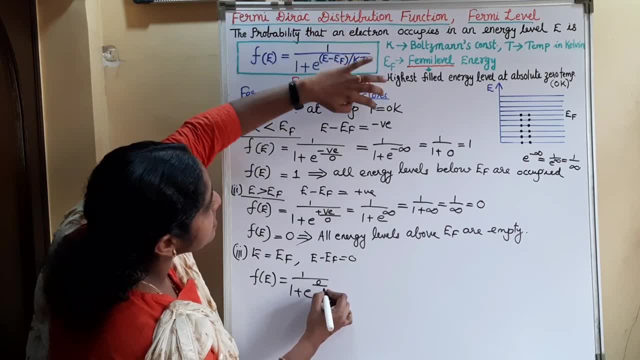 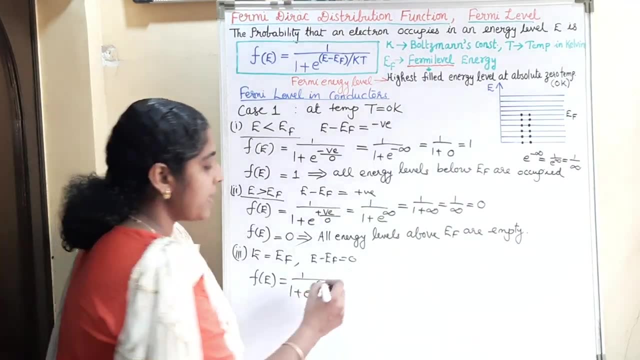 E minus EF is 0, by K is Boltzmann constant, E is 0. That is 1 by 1 plus E raised to 0 by 0. What is 0 by 0? Not defined. So that means this is indeterminate. So if we consider the energy, 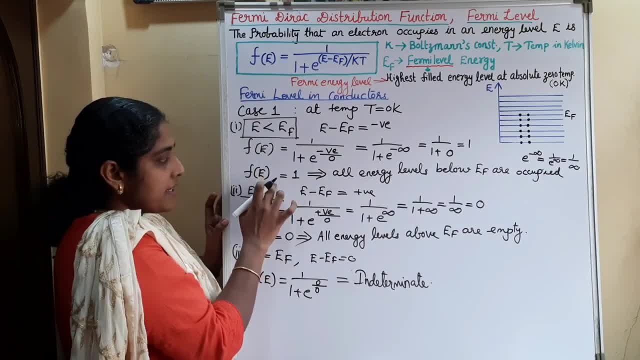 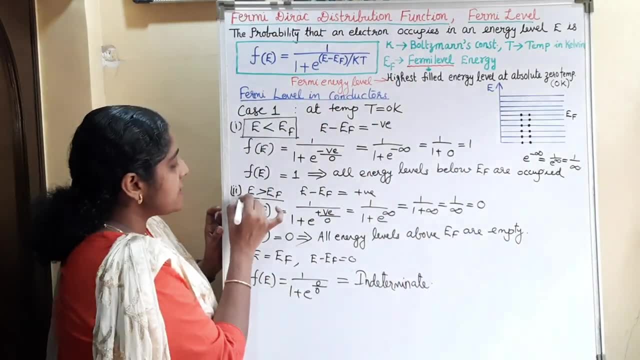 levels below the Fermi level, Fermi direct distribution function is 100 percentage. That is, all the energy levels below Fermi level is completely occupied. And if we consider the energy levels above Fermi level with, the Fermi direct distribution function is 100 percentage. 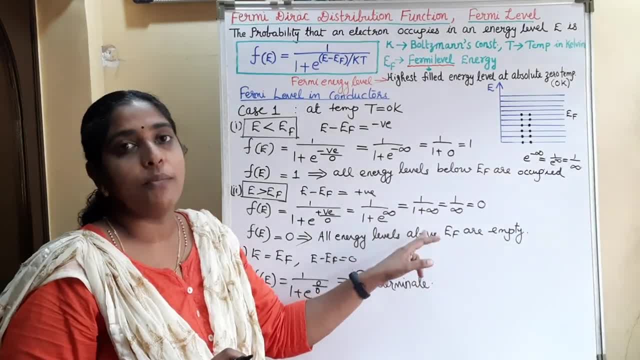 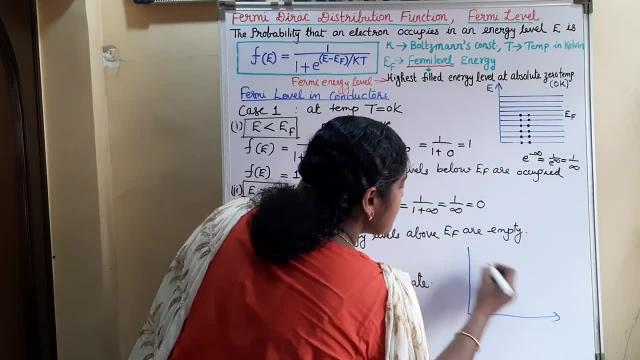 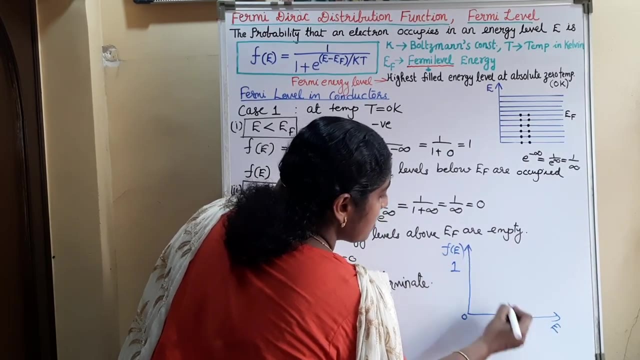 The Fermi direct distribution function is 0.. That is all. the energy levels above Fermi level are empty. So if we draw a graph of F of E versus energy, that is 0.. Here it is 1.. Here we can. 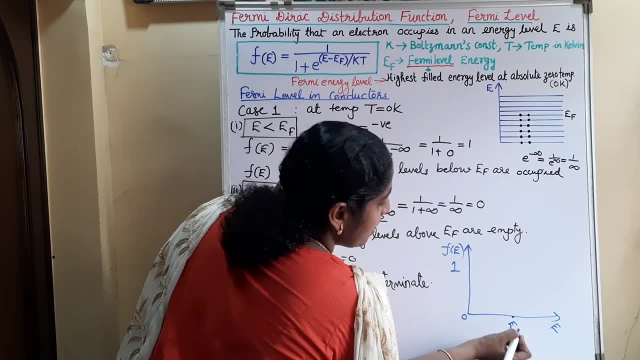 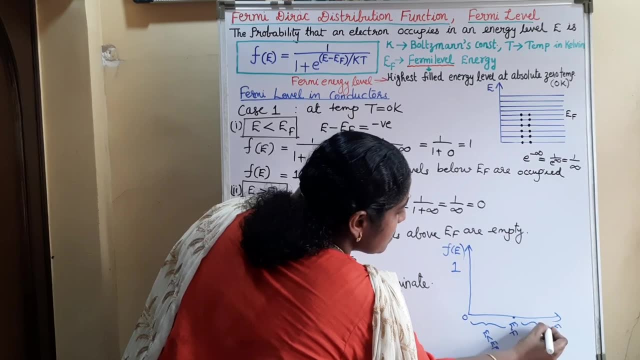 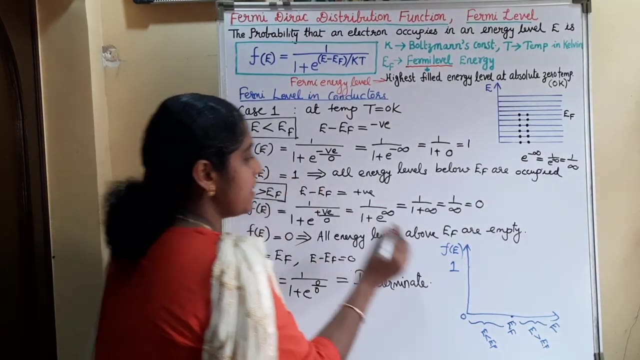 consider an energy level E for EF. So these are the energy less than EF. Here the energy is greater than EF. So these are the energy less than EF. Here the energy is greater than EF. So these are the energy less than EF. When we consider the energy levels below Fermi level, F of E is equal. 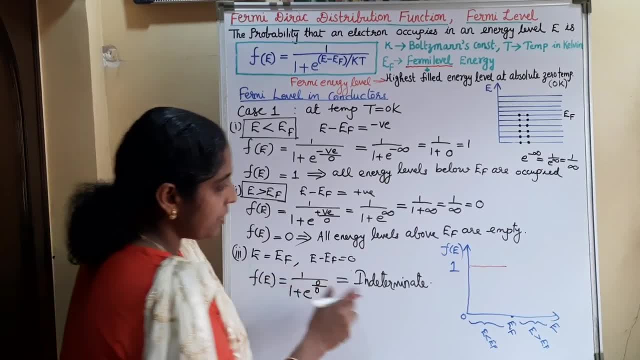 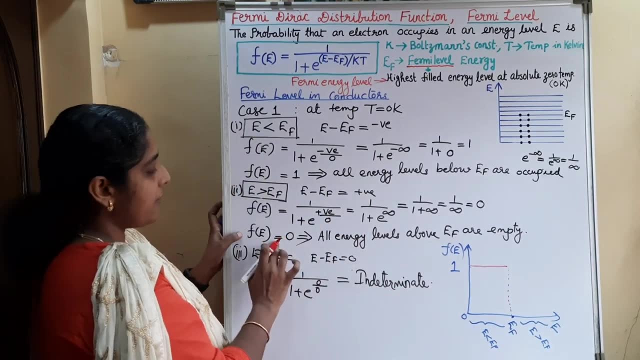 to 1.. So we can consider like this: At E equal to EF, it is indeterminate. And if E greater than EF, then the F of E is equal to 0. That is, we are getting a step-like function, The Fermi direct. 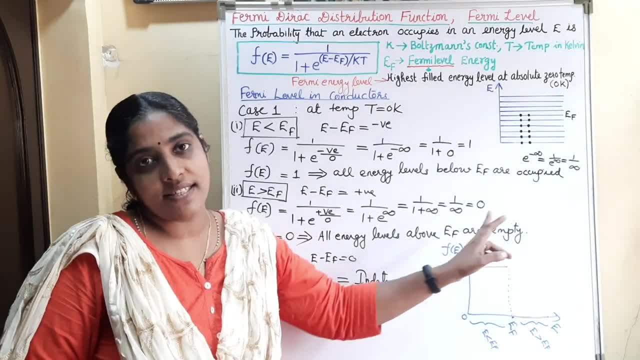 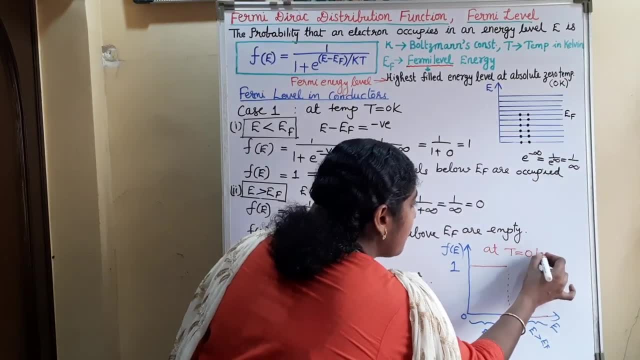 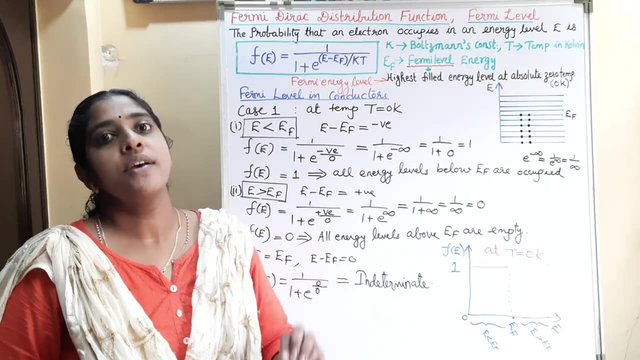 distribution function with the energy levels varying like a step-like form. So here we are considering the condition at T equal to 0 Kelvin, That is, all energy levels below Fermi level are occupied and all energy levels above Fermi level are empty. So for conductors at T equal to 0, 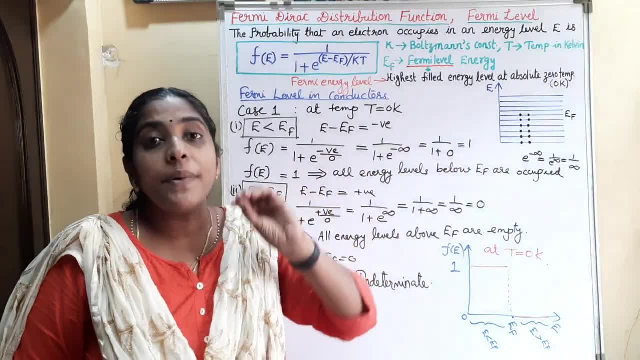 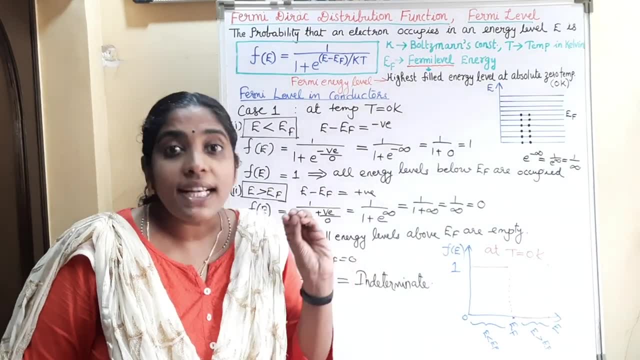 Kelvin, we can define the Fermi level as the uppermost filled energy level, And Fermi energy is the maximum energy of the electron sin conductor at T equal to 0 Kelvin. If we change the condition, that is, as temperature increases, then the Fermi level is the maximum energy of the. 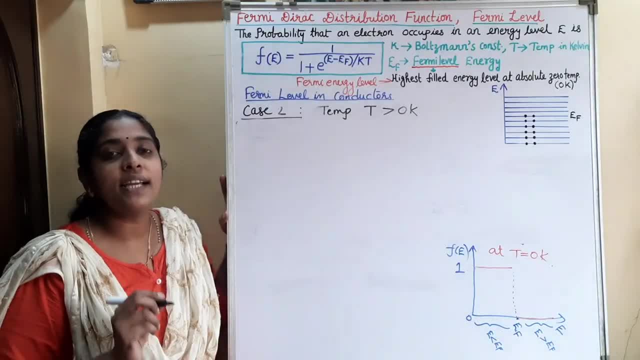 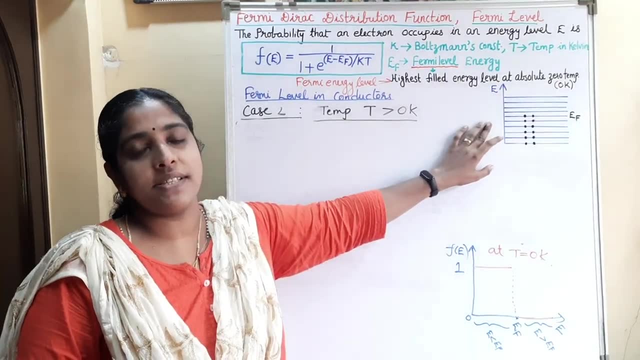 electron. If the temperature increases, the Fermi level definition also will change. Now we can consider the second case, that is, temperature T greater than 0 Kelvin. So what happens as the temperature increases? When the temperature increases, the electrons in the lower energy. 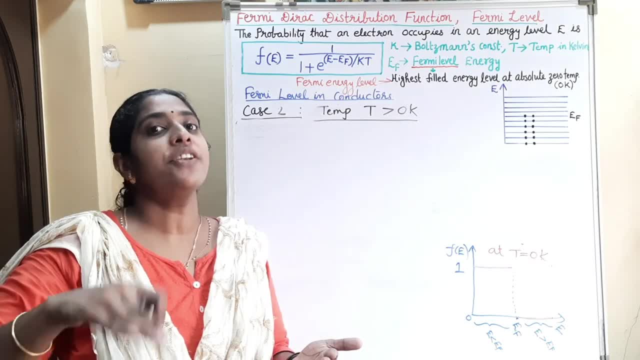 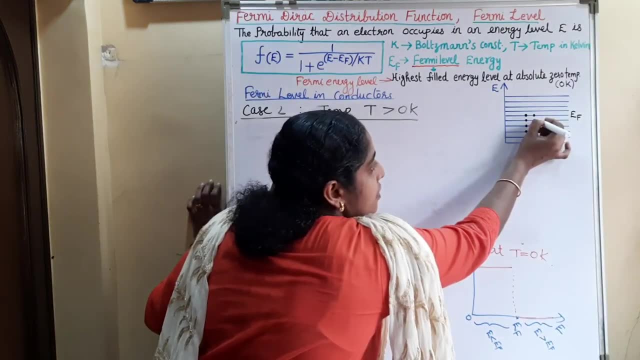 level will get thermal energy and they will excited to the higher energy levels. That is, thermal excitation of electrons will happen. Therefore, this electron from the lower energy level will go to the upper energy level. So the thermal excitation of electrons will happen. So 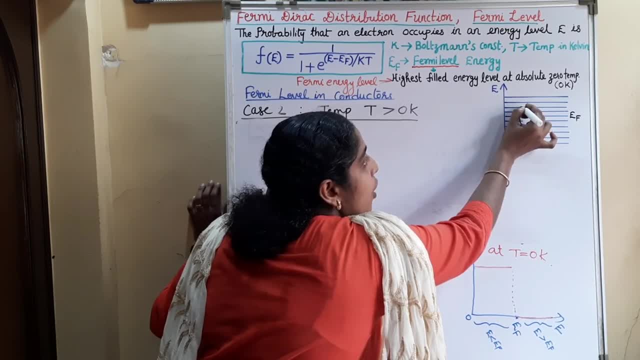 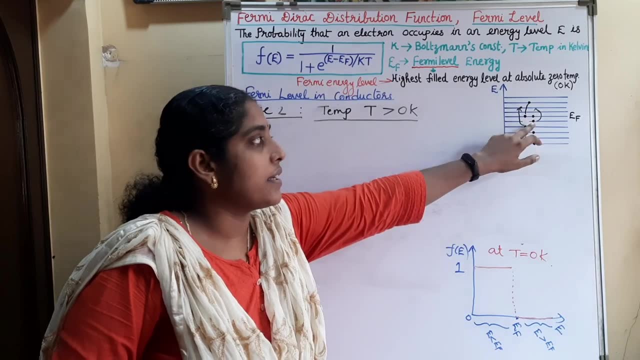 the thermal excitation of electrons will happen. Therefore, this electron from the lower energy level will go to the upper energy level. So the probability of occupancy of electrons in the upper energy level will increase and the probability of occupancy of electrons in the lower energy level will decrease. 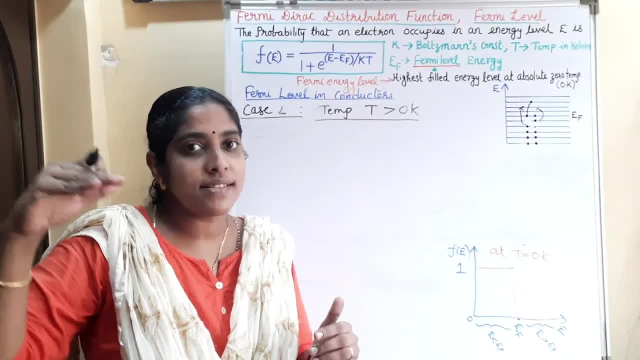 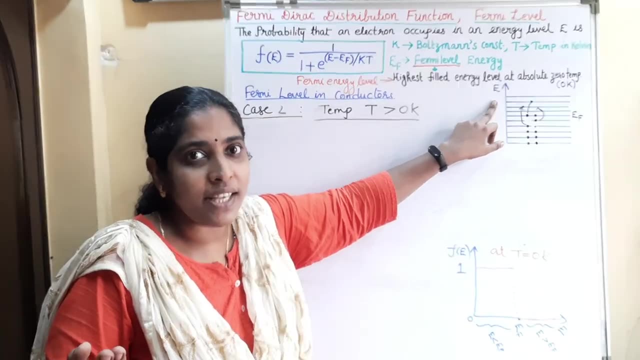 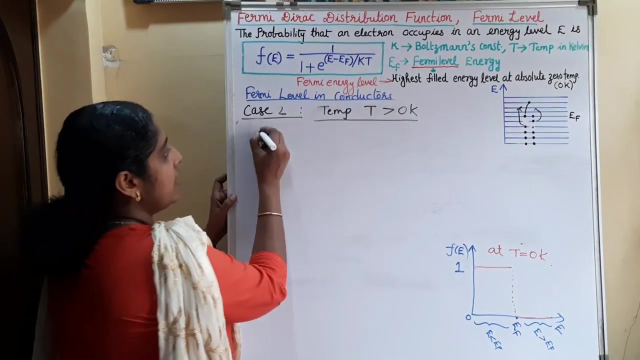 Because as temperature increases, the electrons are thermally excited for the higher energy levels. When the electron will go to the higher energy level, the probability of occupancy of electrons is increasing And probability of occupancy of electrons in the lower energy level is decreasing. So here we can consider a case when E is equal to Ef. So that is. 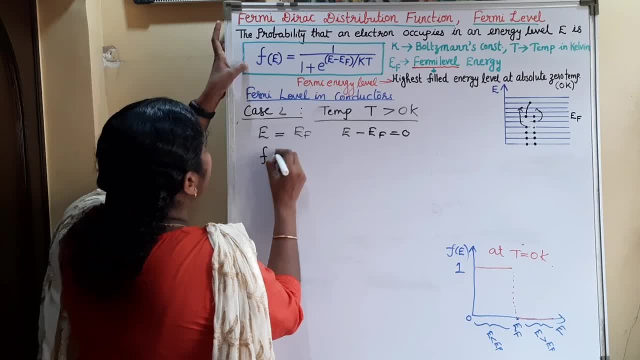 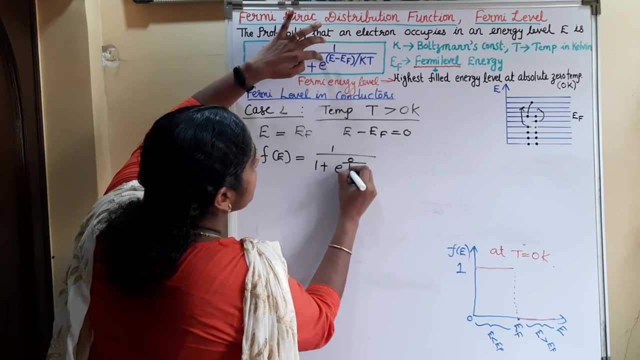 E minus Ef is equal to 0. So this equation becomes: f of E is equal to 1 by 1- True or plus. e raised to e minus ef is 0 divided by kt. here t is greater than 0 kelvin, so it is 1 by. 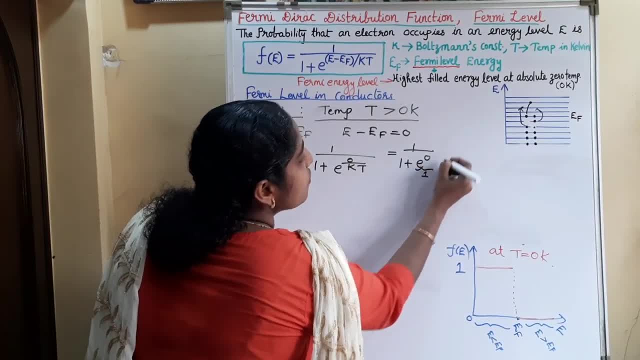 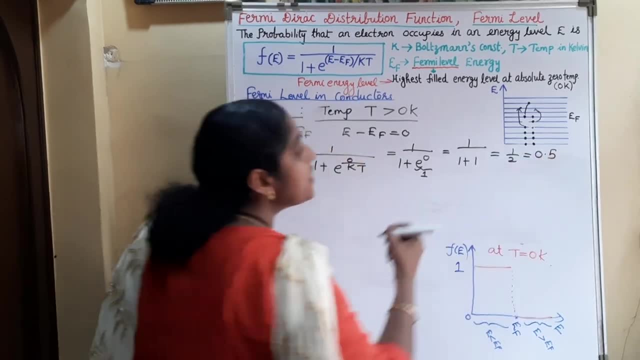 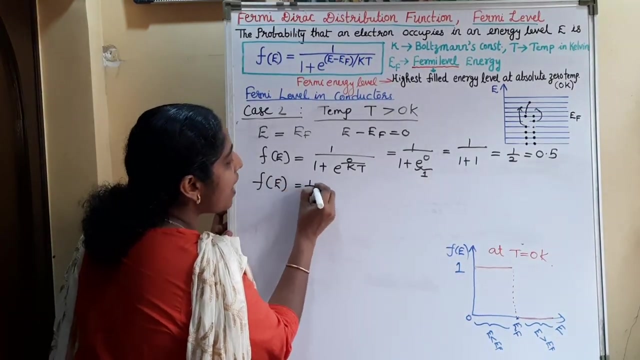 1 plus e raised to 0. what is e raised to 0? 1, that is 1 by 1 plus 1, that is 1 by 2, that is 0.5. that is 50 percentage. so when the temperature is greater than 0 kelvin, f of e is equal to half. 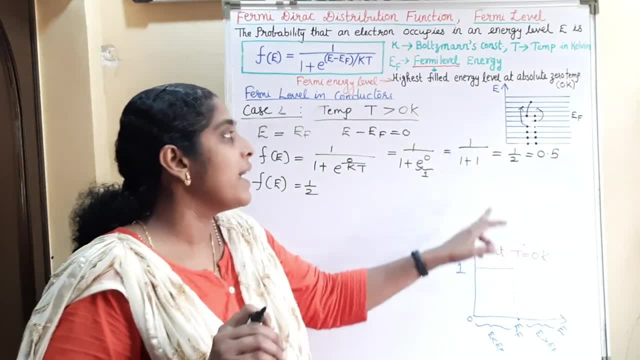 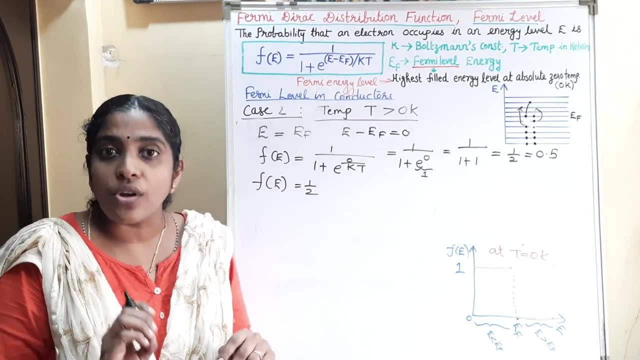 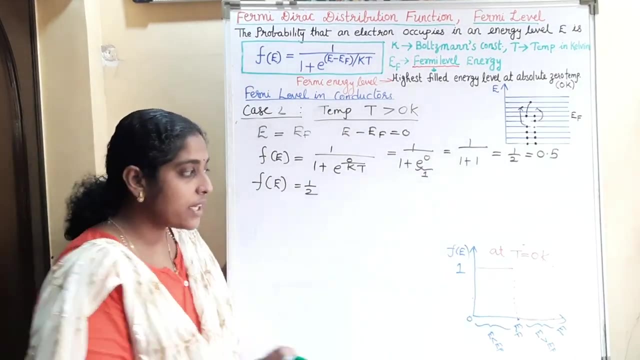 that means there is 50 percentage probability of electrons at the fermi level. so when the temperature is greater than 0 kelvin, fermi level is not the uppermost filled energy level. fermi level may or may not be filled. so while we draw the graph of temperature greater than 0 kelvin, 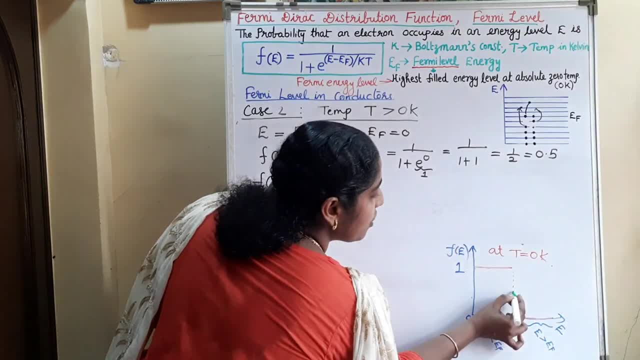 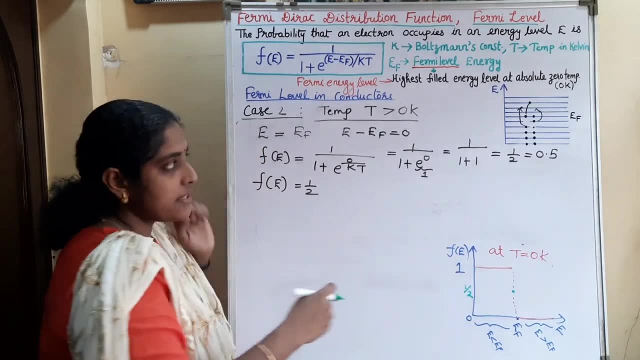 this step, like nature will change. because at a equal to ef, this probability is half. and for the e less than ef, that is the e less than ef, that is the e less than ef, that is, the energy levels below the fermi level, the probability of occupancy is decreasing. so the graph is not.